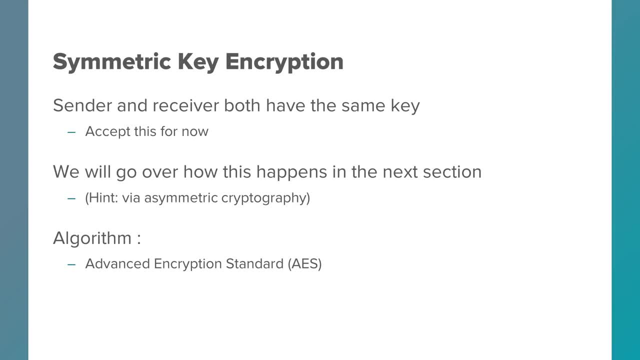 the same private key to either encrypt a message or decrypt a message. You have the sender and the receiver both using the same private key to either encrypt a message or decrypt a message. An example of this symmetric key algorithm is AES, or also known as Advanced. 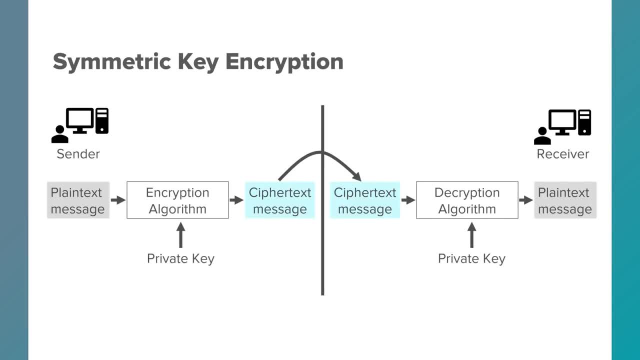 Encryption Standard. Now, the way symmetric key encryption works is on the sender side. it has the plain text message and a private key and it feeds those two pieces of data into an encryption algorithm And the resulting operation outputs a ciphertext message And. 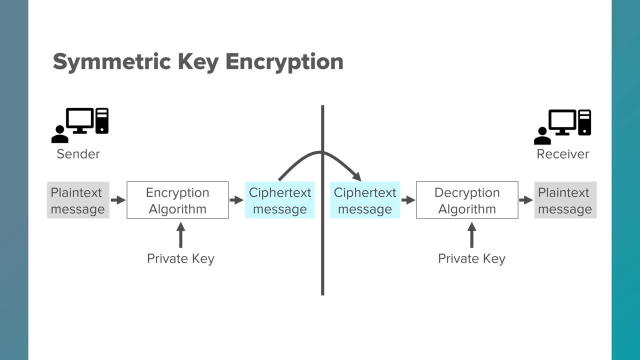 this ciphertext message is what gets sent over to the receiver. So when the receiver is ready to read the message, they take the ciphertext message and use this as input to a decryption algorithm. The receiver also gives it as input the same private key that the sender has used to encrypt this message. And when the receiver runs this, 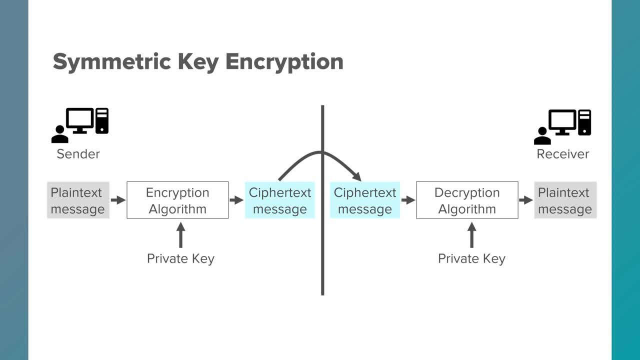 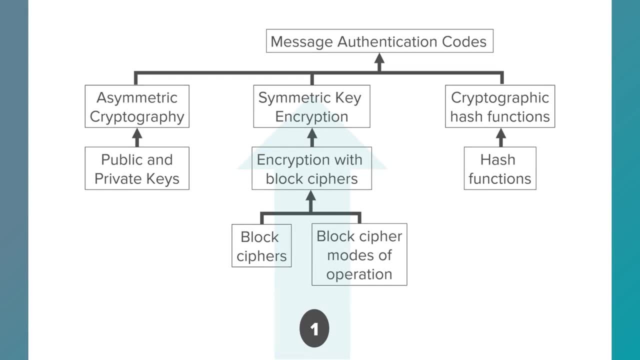 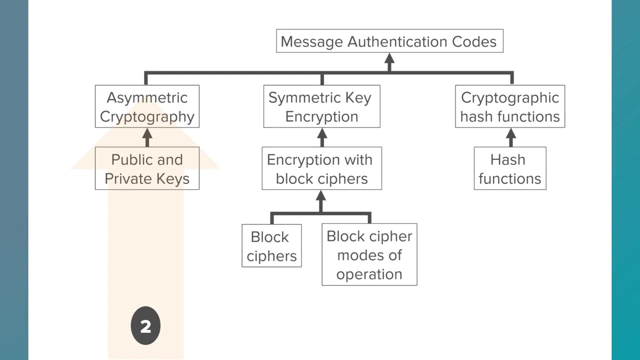 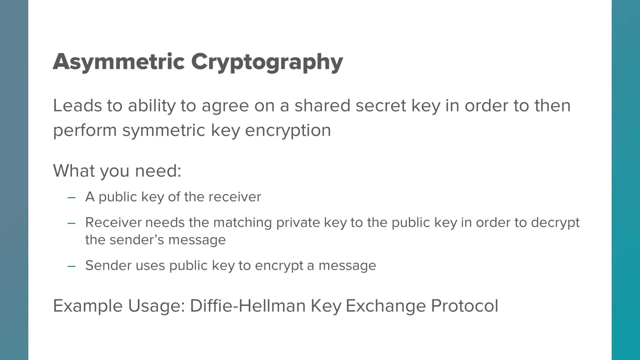 decryption algorithm process. the output is a plain text message that the sender intended to send to the receiver. So now we just looked at symmetric key encryption. Now we'll move on to introducing asymmetric cryptography and mention public and private keys. Asymmetric cryptography is that concept that leads us to having the ability to agree on. 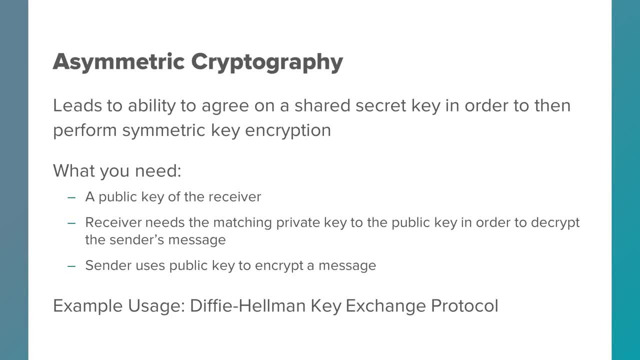 a shared secret key, And that shared secret key is then used to perform symmetric key encryption. Now, in asymmetric cryptography, what the sender needs is a public key of the receiver which is used to encrypt their message to the receiver. The receiver needs the matching private key to that public key in order to decrypt the sender's. 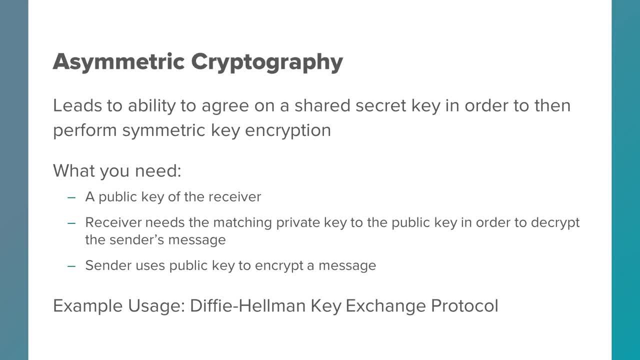 message Effectively during asymmetric key encryption. the message is the agreed-upon symmetric private key that the sender would like the receiver to use in future symmetric key encryption processes. An example of this key exchange protocol is Diffie-Hellman. So now, 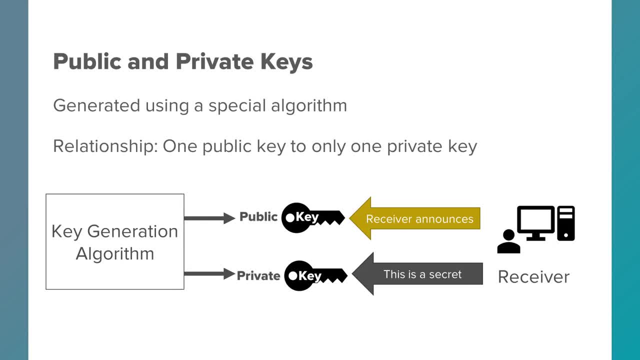 let's move on to talking about public and private keys in a little bit more detail. Public and private keys are generated using a special algorithm, a key generation algorithm, And the relationship between the public and the private key is that there's only one private key.